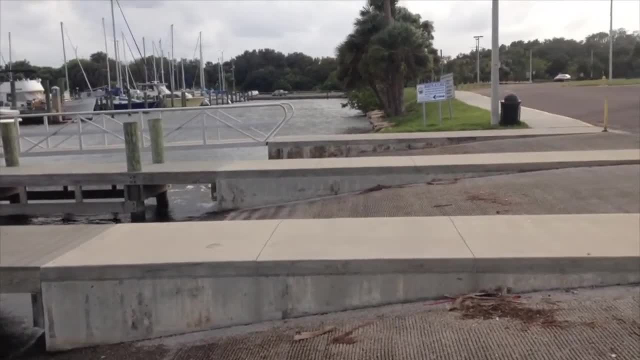 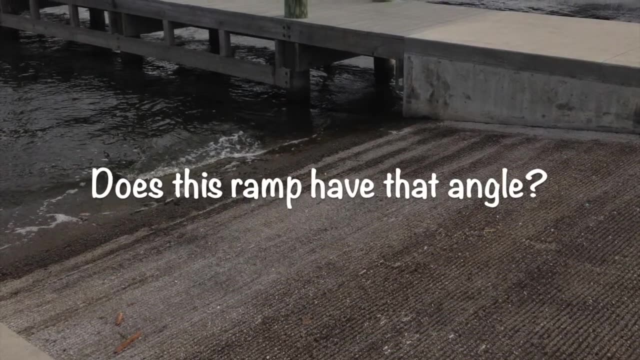 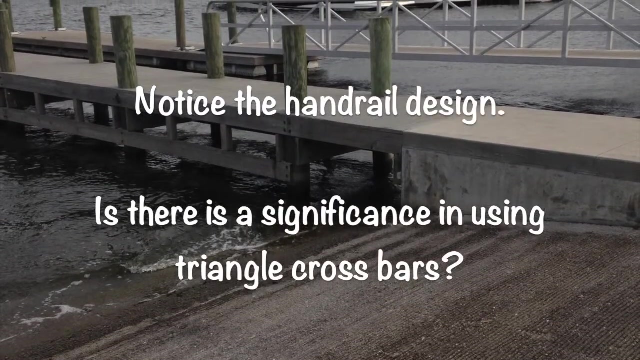 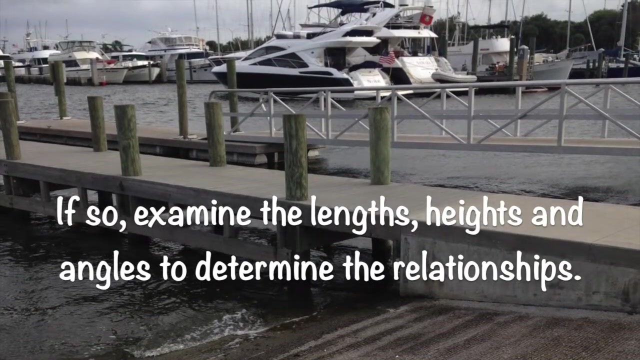 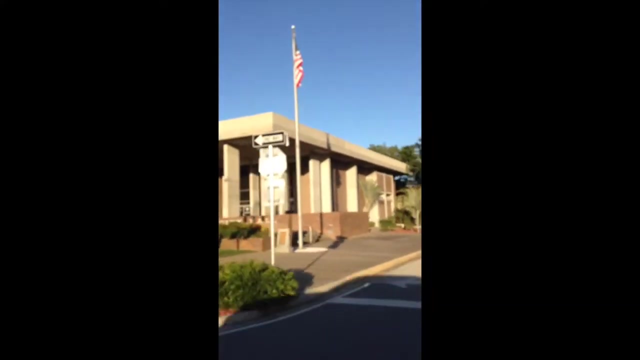 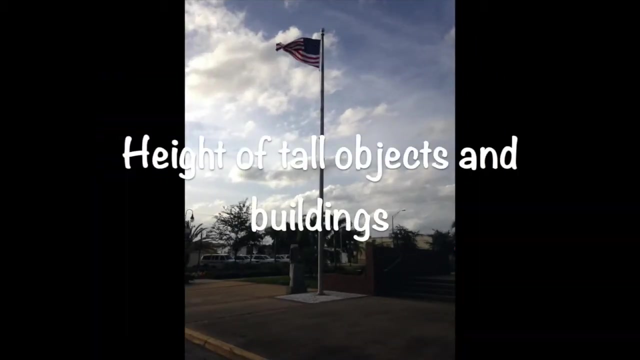 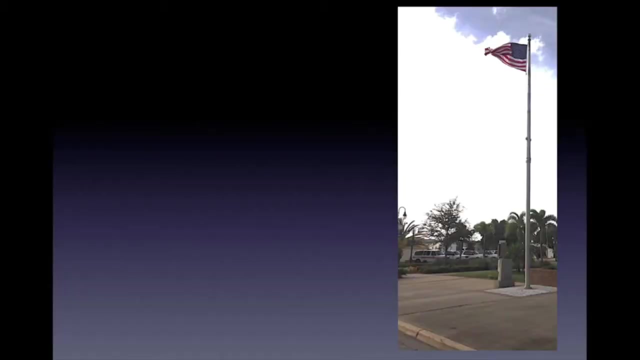 Thank you. I'm going to find the height of a flagpole I found on my drive. First I'll find the distance I'm standing from the base of the flagpole. Next I'll calculate the angle of elevation from where I'm standing. 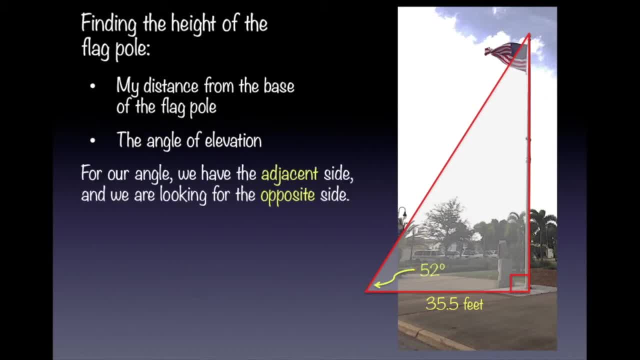 looking to the top of the flagpole, For our angle we have the adjacent side and we're looking for the opposite side, which represents the height of the flagpole. The trigonometric function we'll use is tangent, since it represents the ratio of the opposite side to the adjacent side. 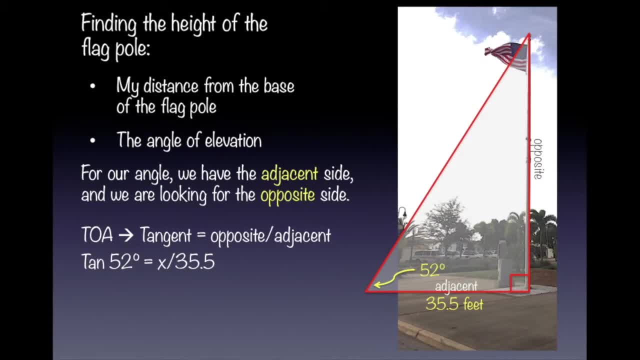 So tangent of 52 degrees is equal to x, our opposite side, or height of our flagpole over 35.5.. Multiplying both sides by 35.5, to get x by itself, we have x equals the tangent of 52 degrees times 35.5.. 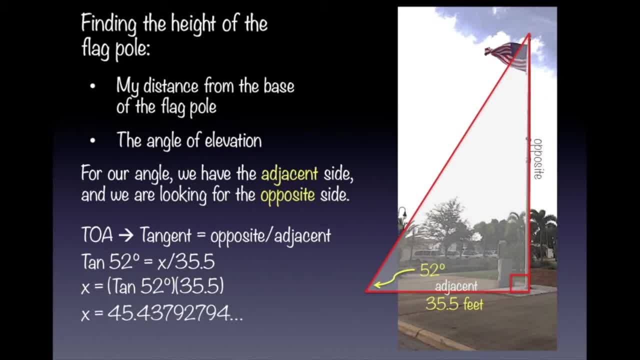 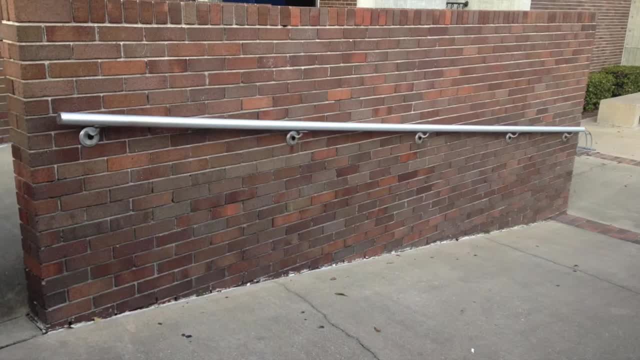 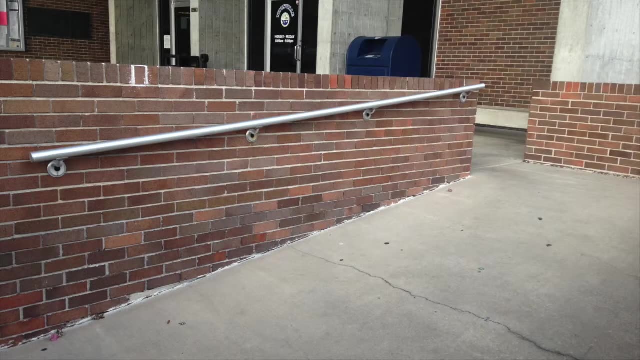 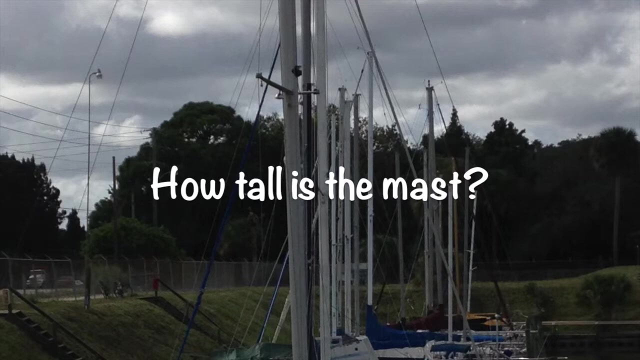 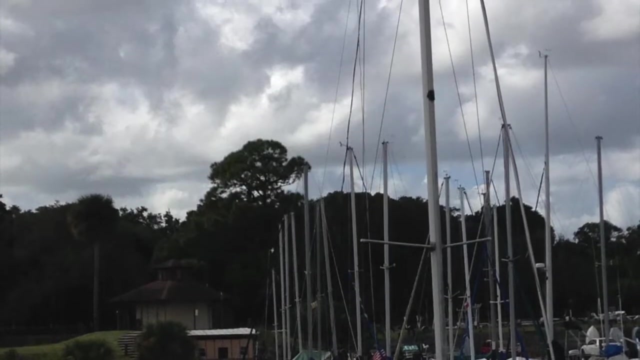 Using a scientific calculator. we perform the calculation and find that the height of the flagpole is approximately 45 feet. If we look closely at x- at 35,, we'll notice that x equals x. This is nothing unlike our initial нат 이상 height. 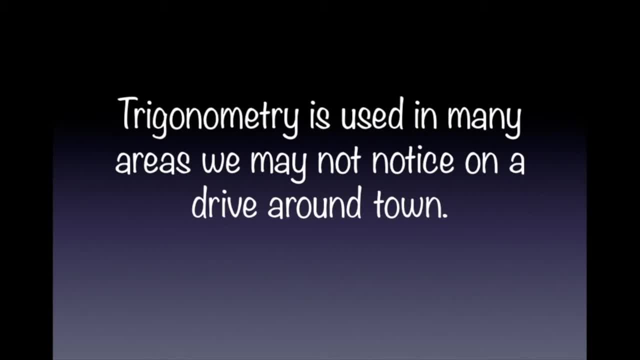 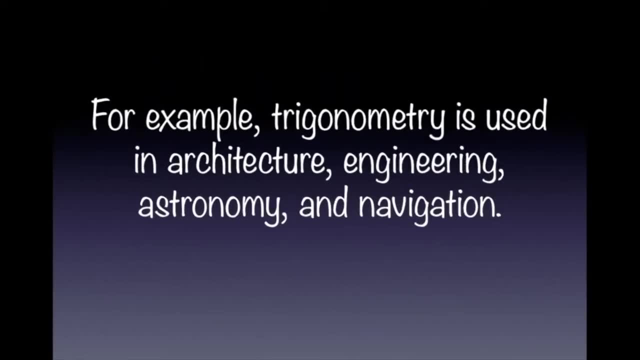 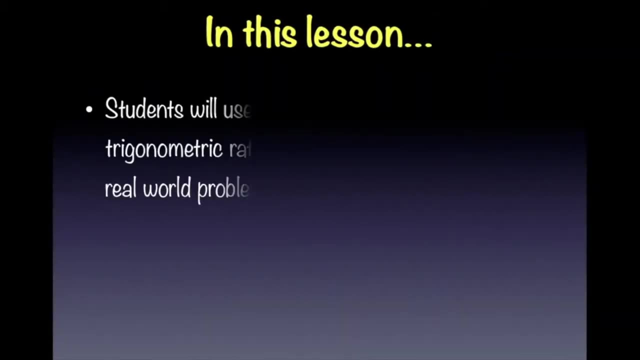 In this example, shipping agent. y equals the intuition of how high 5 gold marks feel saludable. Next I'll calculate the никто standings of exactly which point x equals x. In this lesson, students will use trigonometric ratios to solve real-world problems.